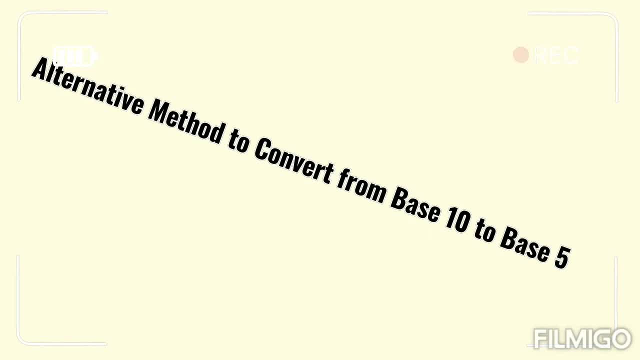 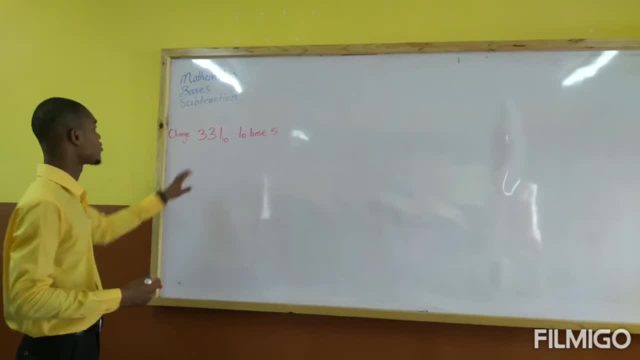 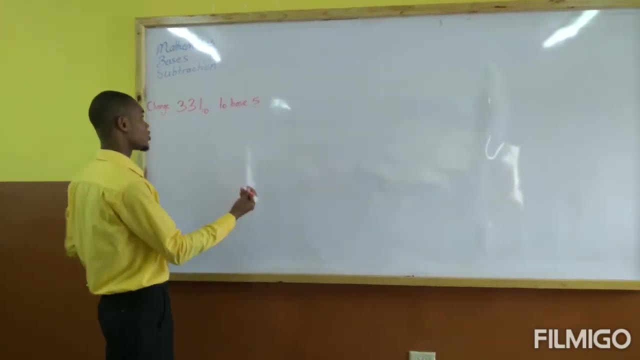 Alright, welcome back Mr Raul here. So we are doing an alternative method to convert from a step to a stack. So you would have done another method before, but this is another way to do it. So what you write, you put here a number that is supposed to be converted. 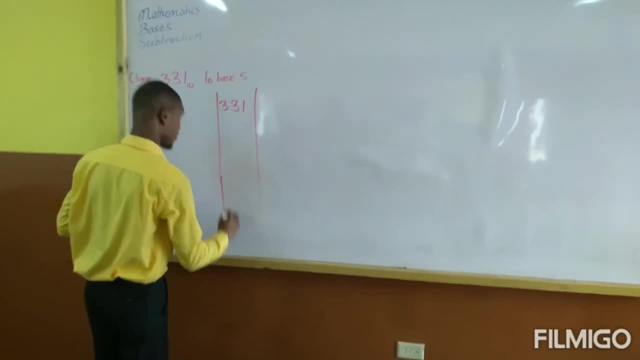 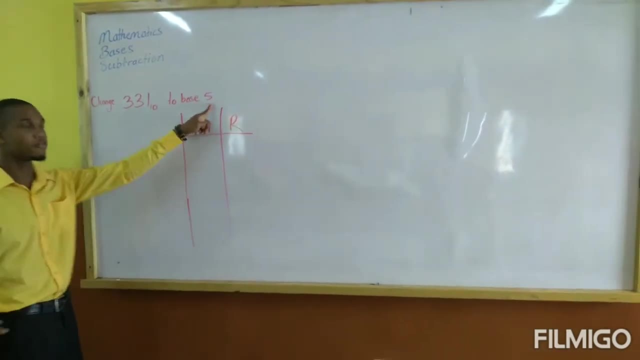 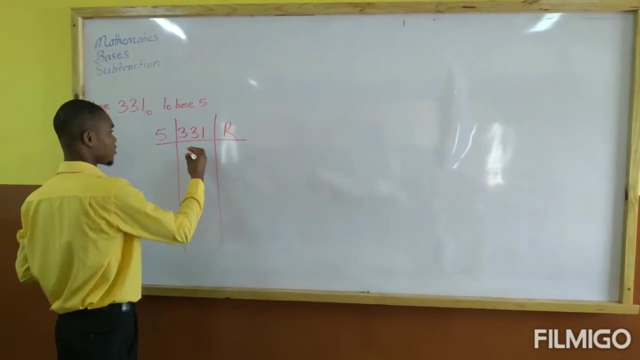 You draw lines around it, You put the letter R here, which means remainder, And you put the base that you are converting to over here, And then you start to divide. So 5 times 3 is 33.. You would work that out and that would be. 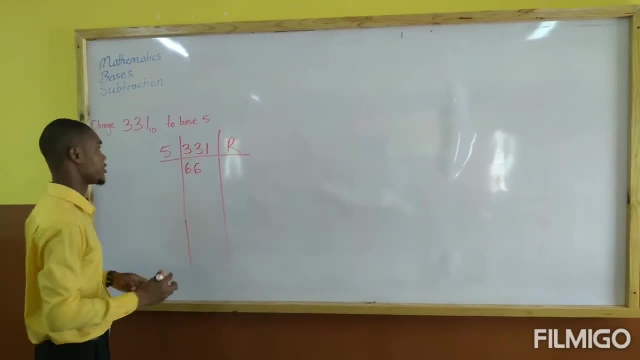 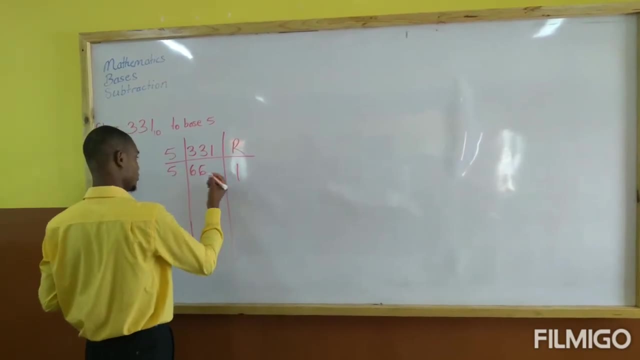 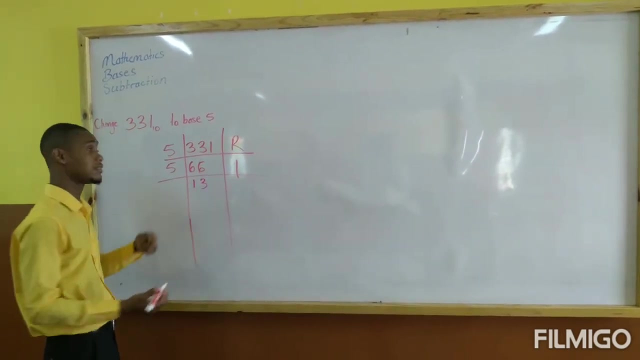 So 66. So 5 times 66 would give you 330. And you put your remainder over here, which is 1.. Then you divide 66 by 5, and that would give you 30. And that, when 5 times 13, is 65, so you would have a remainder of 1 here. 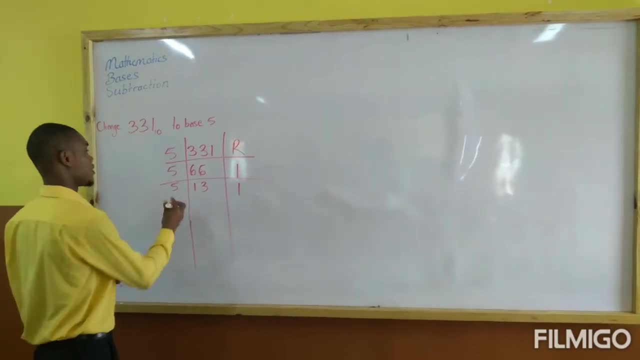 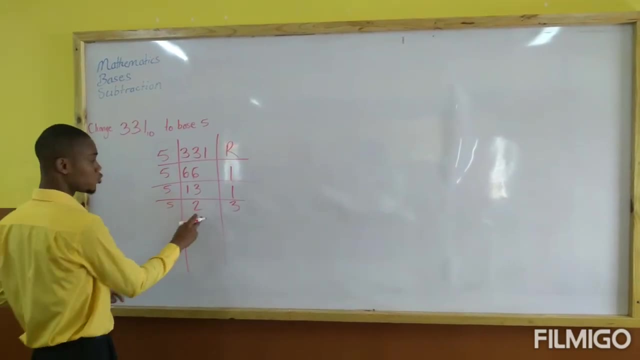 Then you divide 5, 13 by 5.. So 13 divided by 5, that gives you 2.. And you put your remainder over here, which is 3.. 5 into 2, that's a 0.. 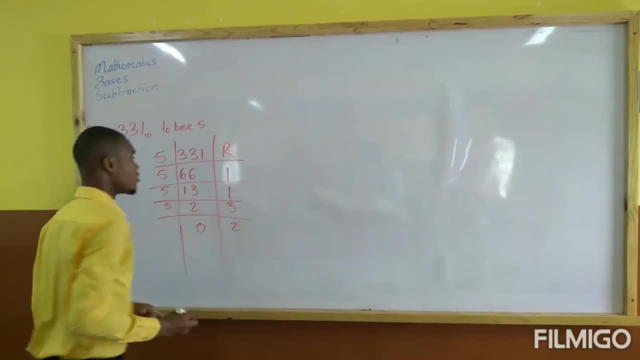 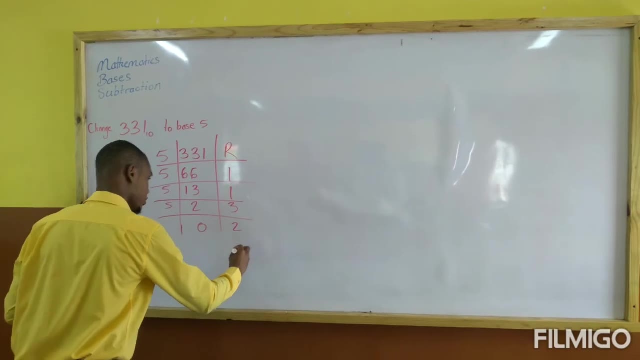 And you would still have a remainder of 2.. So because you have arrived at 0 in the middle, it means you cannot divide up any further. So you put your hands up, Start writing your hands up, from the bottom going upwards. 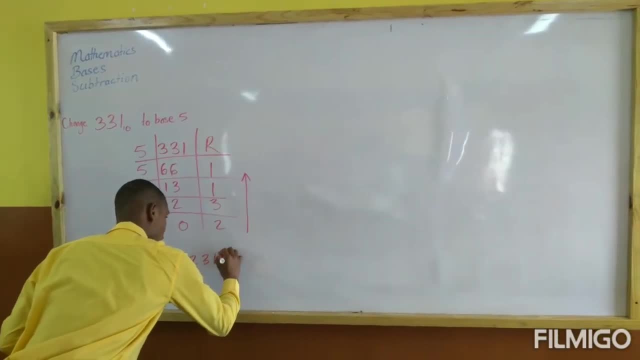 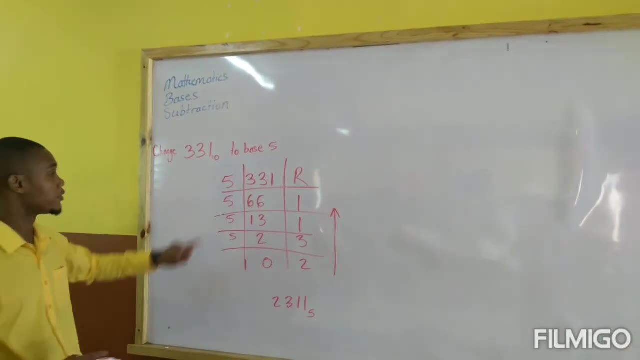 So that would be 2, 3, 1, 1, base 5.. And the reason you write from the bottom going upwards is because of the modules. The more you divide by 5, it means you are dividing up. 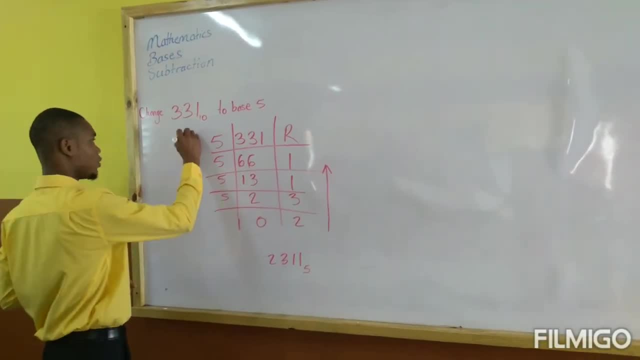 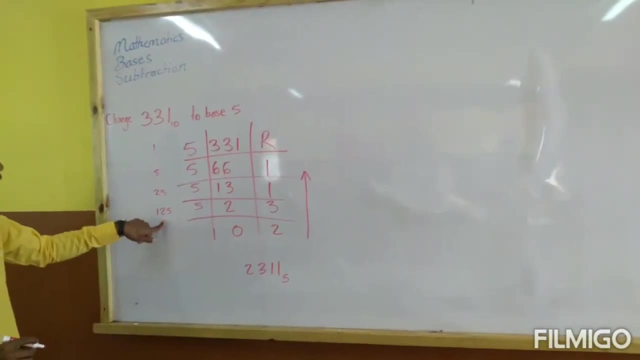 And the entire thing by a larger volume. So this would be 1,, this would be 5s, this would be 25s and this would be 1, 25.. So because this is the largest number to use to divide, it's going to have to be written first. 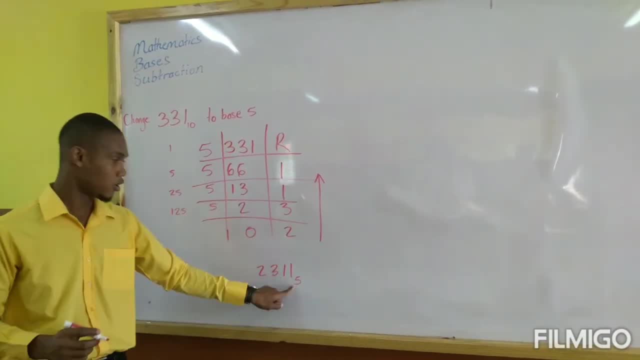 then 25, second, 5, third and then 1s goes last, And that's how we divide, using this method.